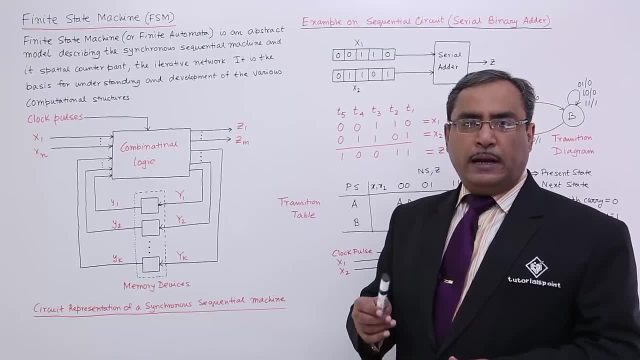 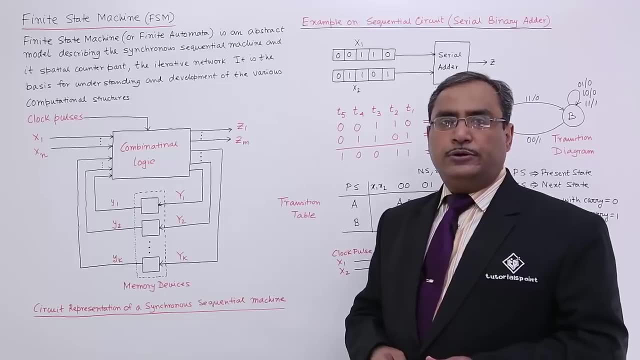 synchronous sequential machine. Synchronous means it will depend upon the clock period or the clock pulse. After application of the clock pulse, something will happen. And sequential machine means we know that all the digital circuits can be divided into two categories: combinational and. 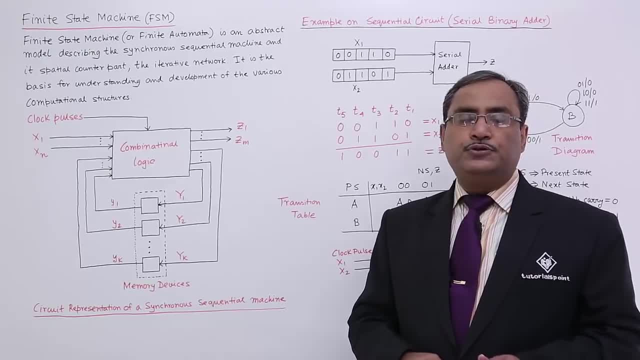 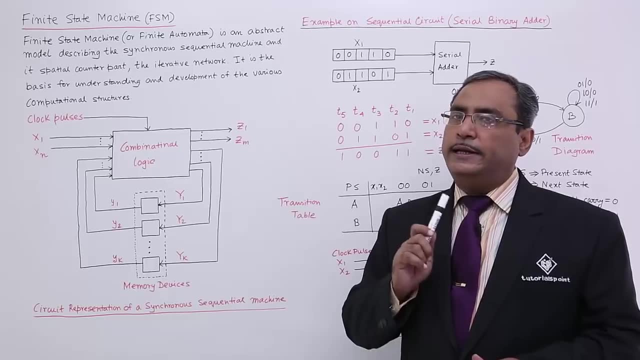 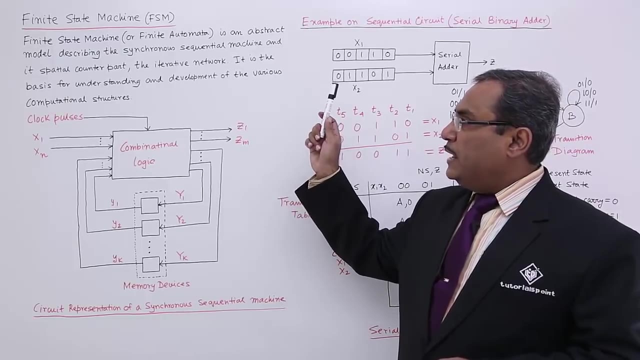 sequential. In case of combinational circuit, inputs will decide the output. In case of sequential circuit, present input and previous output will decide the next output, and that is the sequential circuit. So let us start Describing the synchronous sequential machine and its special counterpart and the iterative. 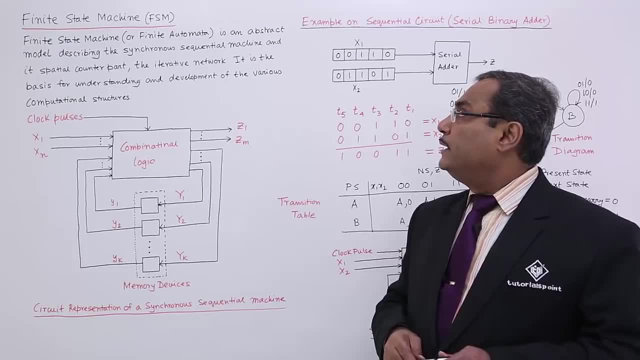 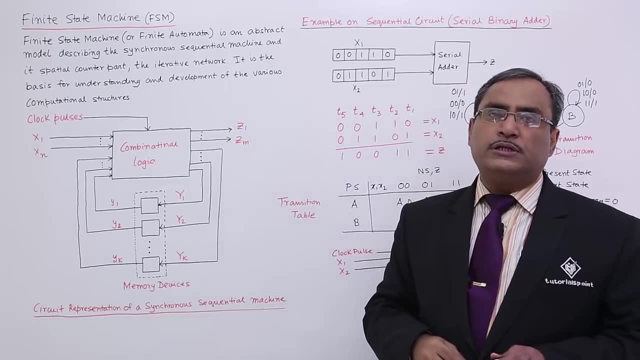 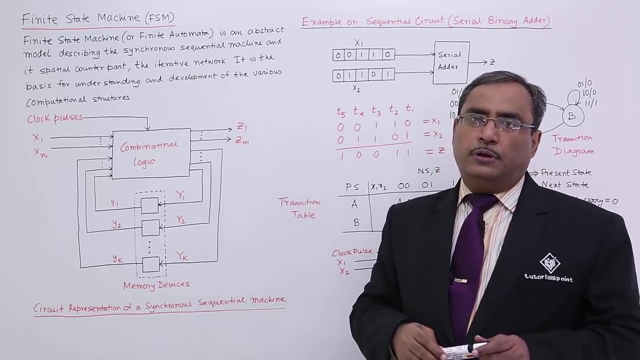 network, So it is having a time dependent phenomenon. It is the basis for understanding and development of the various computational structures, So that is known as the finite state machine. If the definition is not clear to you, let us go for one example that will. 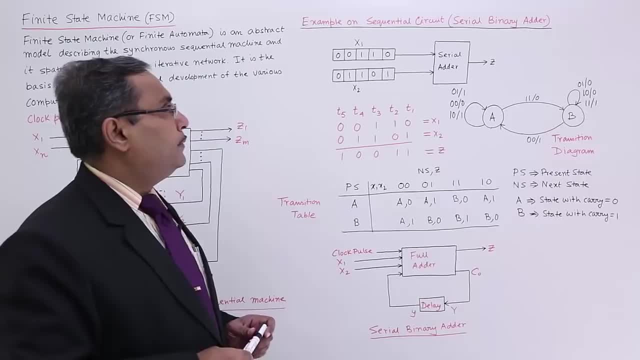 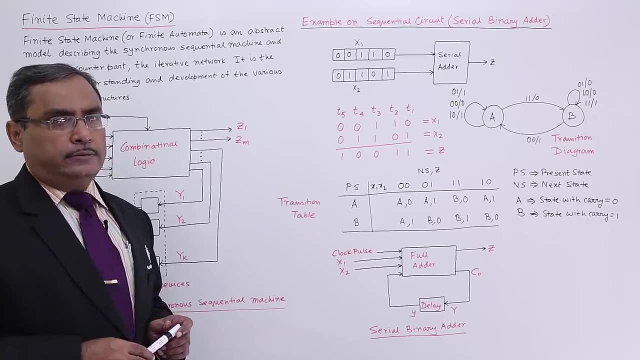 clear your doubts and will give you more clarity on the topic. So let us suppose we are going to discuss sequential circuit, which is serial binary adder. It is a very simple circuit. You might have read this one in your digital electronics classes. 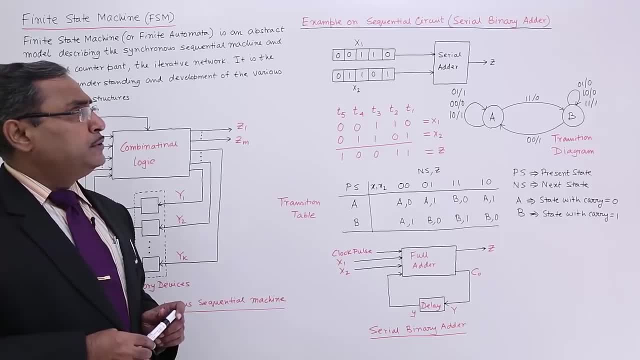 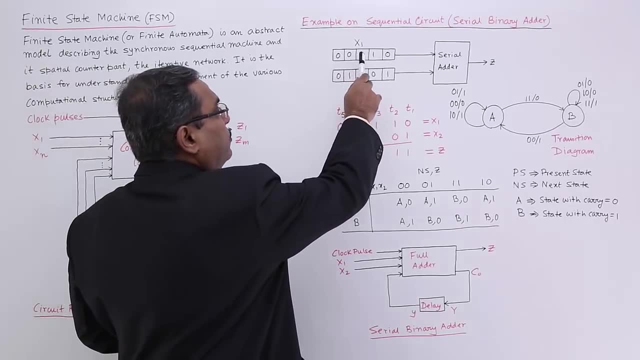 So that is our serial binary adder. Let us suppose we are having two numbers, x1 and x2.. x1 is having the bit pattern like 0, 0, 1, 1, 0, and x2 is having the bit pattern like 0, 1, 1, 0, 1.. Okay, 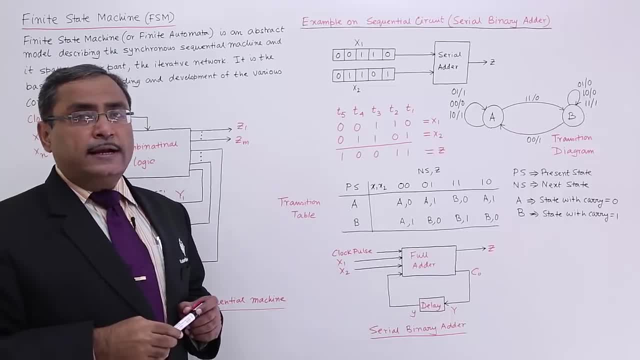 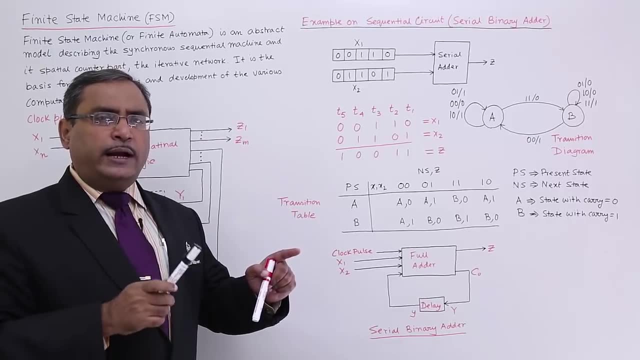 We have taken this one arbitrarily And one serial adder is here. We know the serial adder. That means one input, one bit from x1 will go to the serial adder along with another bit from x2.. These two bits will get added and the output. 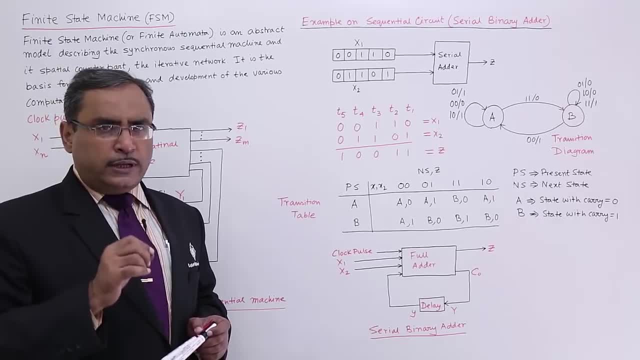 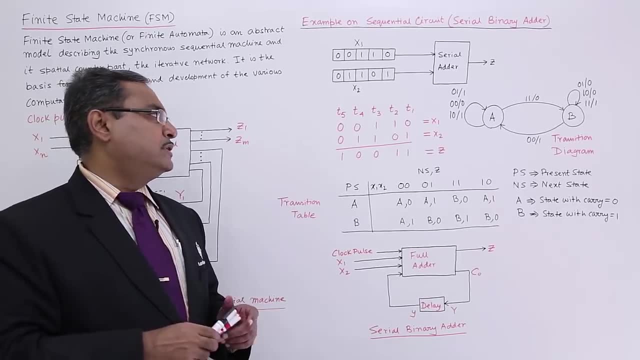 will be obtained and that will be the z. But we know that if we go on adding two bits, obviously the previous carry should be taken into our account. So let us go for such example. So let us suppose this is the bit patterns, Whatever we have taken. 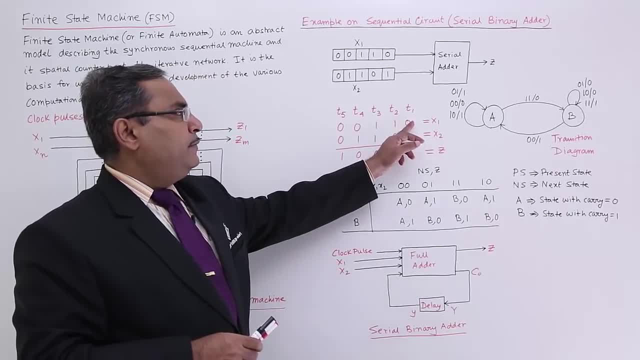 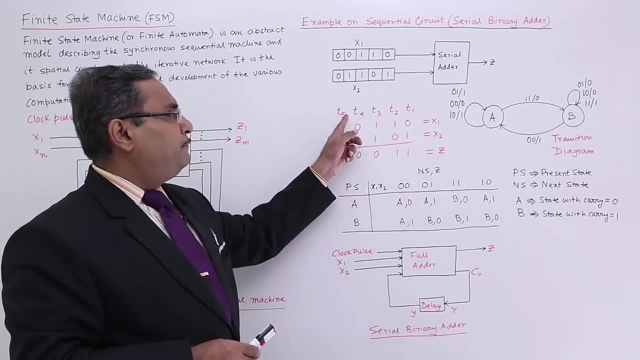 we have written this one here. At t1 instant of time: 0 and 1 will be available there. At t2 instant of time: 1: 0 will be available there. In this way, at t5 instant of time, 0: 0 will be. 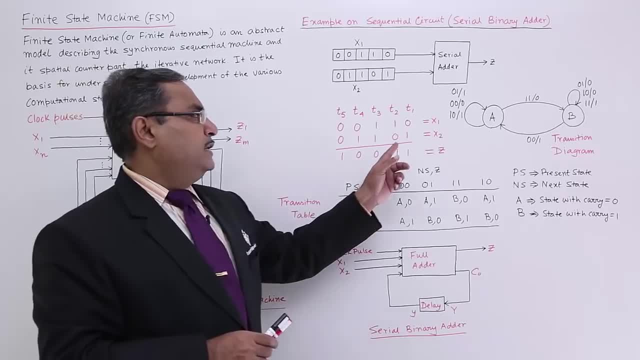 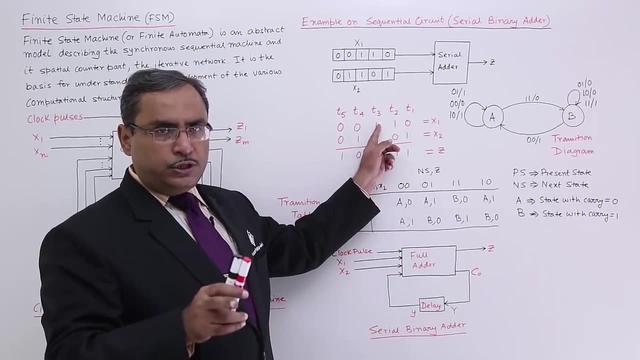 available to the serial adder. Now please go on. adding: 0 plus 1 is 1.. 0 plus 1 means 1.. 1 plus 1 means 2.. 2 means 1- 0. So 0 will be coming, 1 will be the carry And that 1 plus 1 is equal to 2. 2. 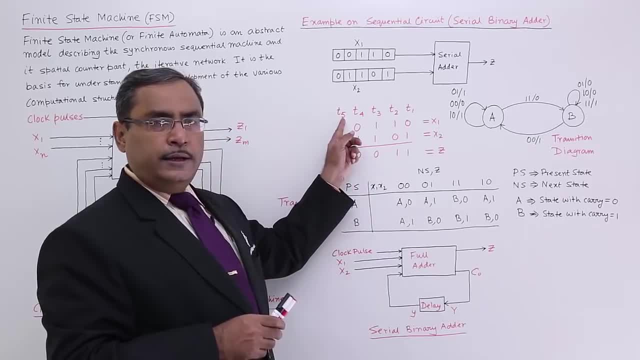 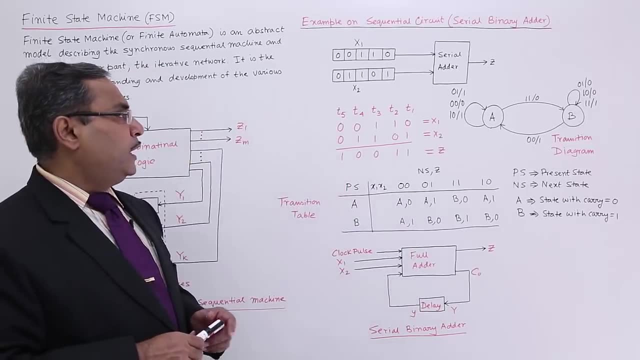 means 1: 0. So 0 will be there, 1 will be the carry, And 1 plus 0 plus 0, it will give you value 1.. So it is a mere binary addition, Nothing difficult here. So in this way the z will be. 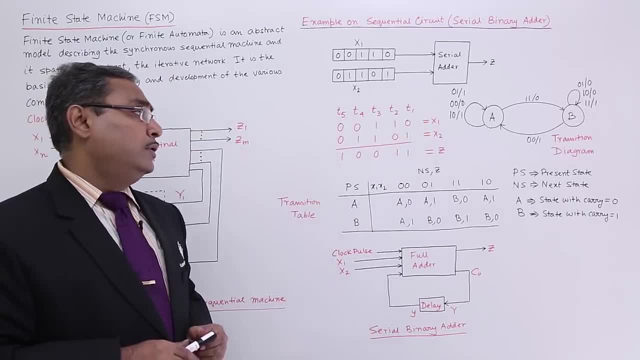 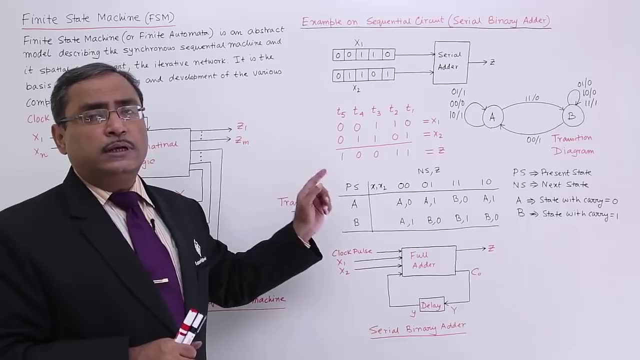 obtained and that is my z. Now I want to represent this particular serial adder. It is a synchronous serial adder. Why synchronous Sequential? Why Because it is sequential. Because not only the present inputs but the previous stage carry will also. 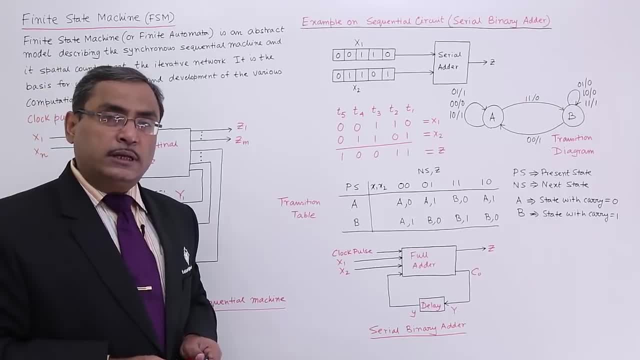 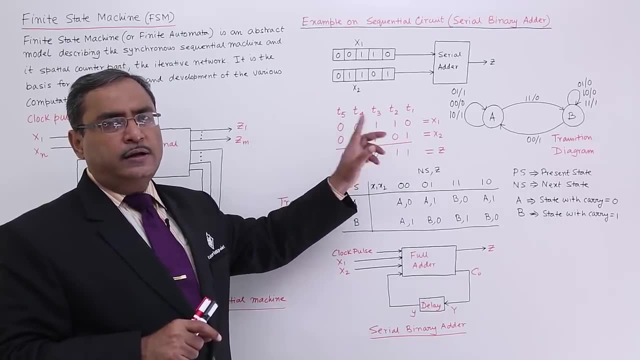 be counted. So that is why it is sequential And why it is synchronous, Because I shall apply 1 clock pulse. Then 1 bit from x1 and 1 bit from x2 will go to the serial adder for the addition. 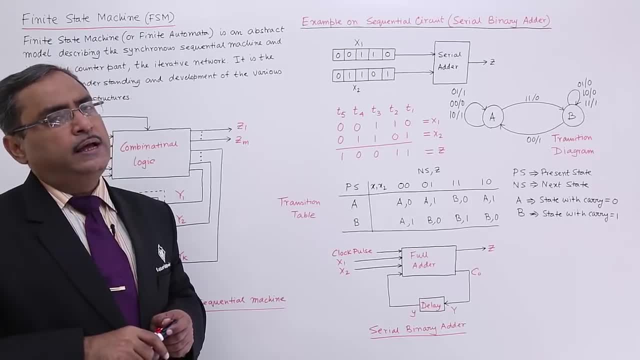 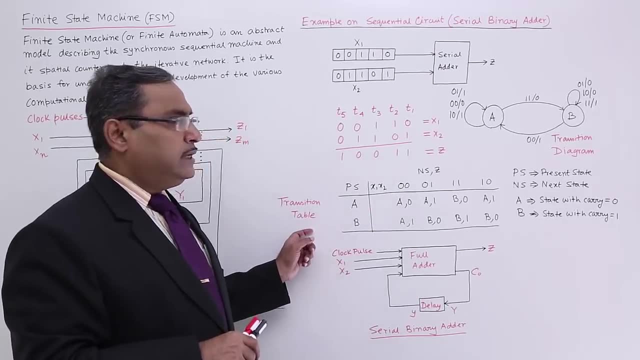 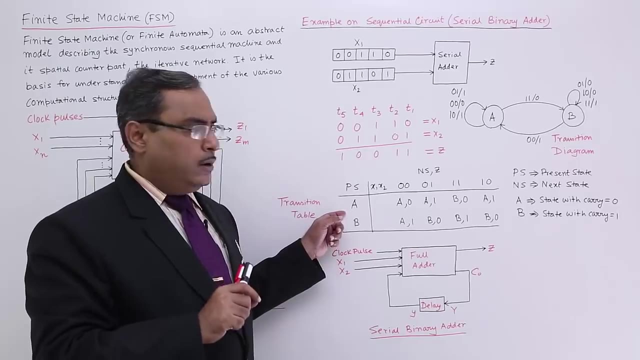 And that addition will also take care of the previous state carry. So that is why it is synchronous and sequential. See, this is my transition table. What is A? A means that very state of this serial adder with the carry 1.. Sorry, 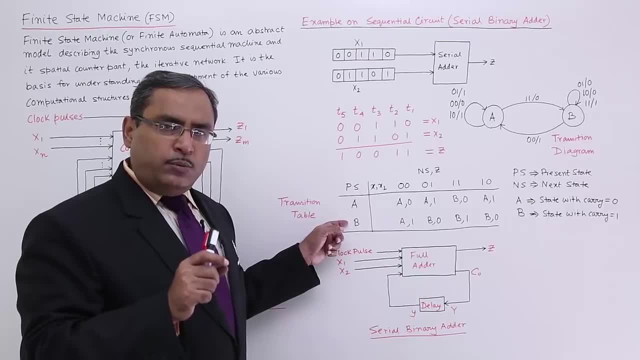 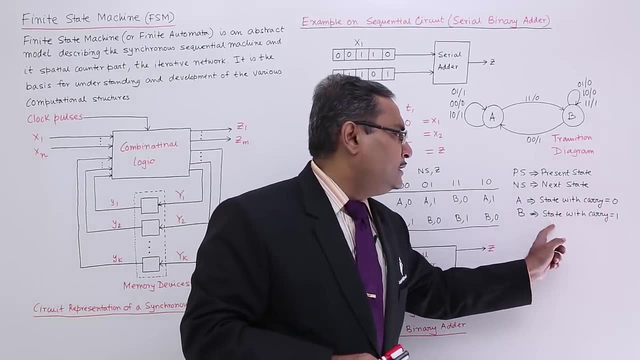 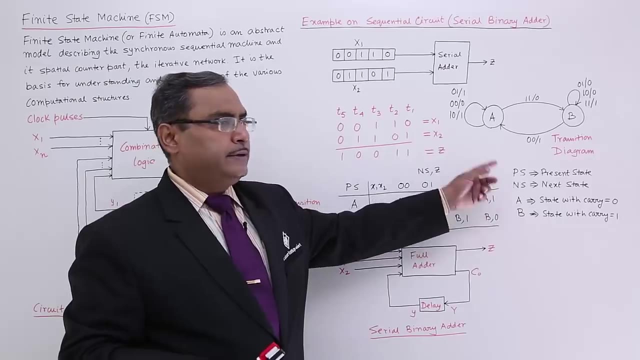 the carry 0.. Sorry, In case of B, what is B? That is the one of the states of this particular serial adder with carry 1.. Everything has been written here: State with carry 0 and state with carry is equal to 1.. So A and B, And you know that is my next state and this is my present state. 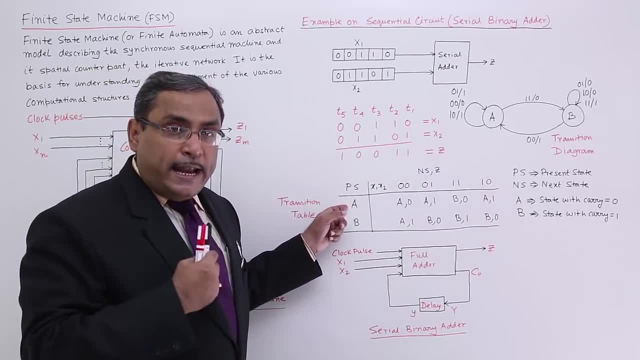 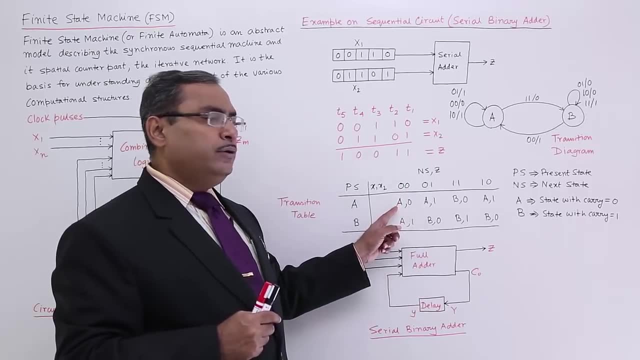 See, if I am at the state A, that means my previous carry is 0. So now, if I get 0, 0, then I shall be in some state A. Why? Because there will be no carry generated and the sum will be 0. So 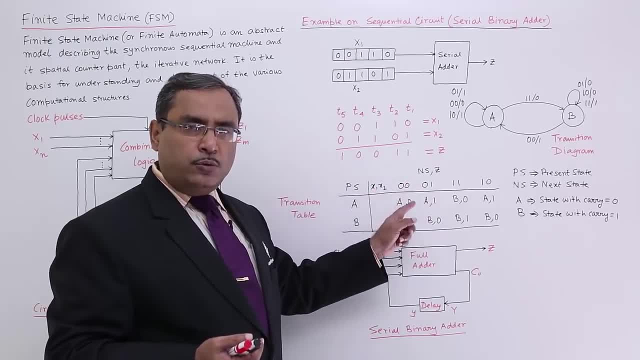 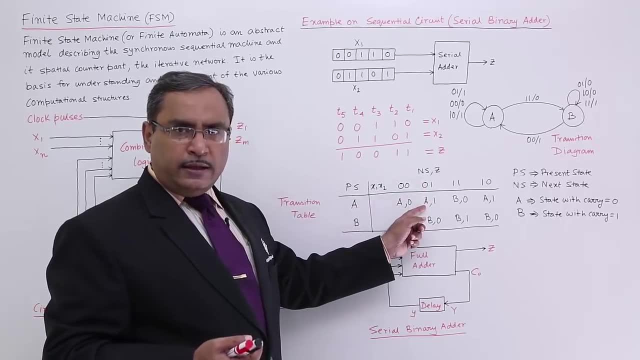 01.. So 01 means actually I am doing 0 plus 0 plus 1, because previous state carry is 0 and here is 01.. So I shall be in a state A without any carry. So that is why I will be in state A and with the. 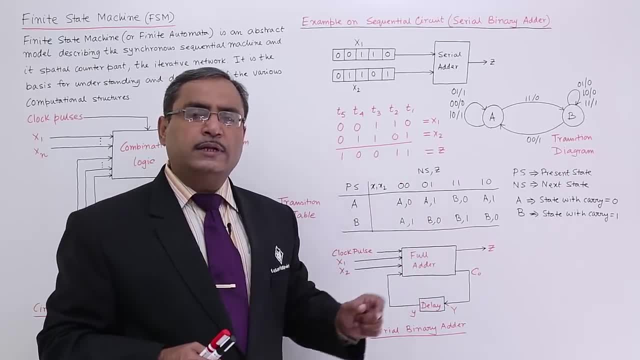 sum 1. So 1: 1. So 0 plus 1 plus 1.. What is that? That is 2.. 2 means what? Means 1: 0.. Means that some and some is less than or equal to 1. So 0 plus 1 plus 1.. So that is 2.. 2 means what? 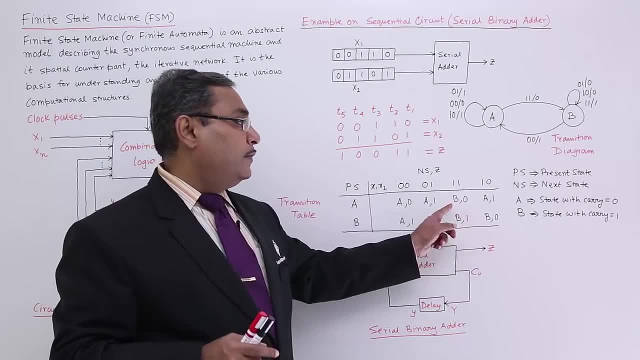 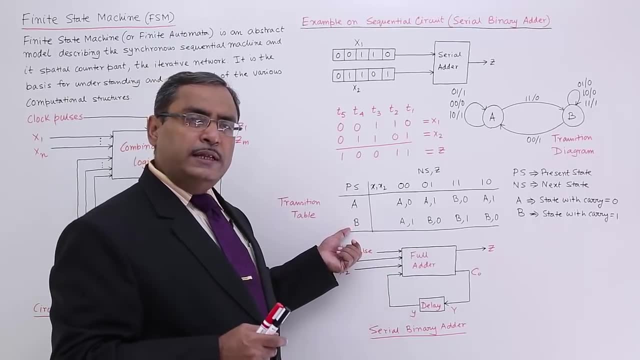 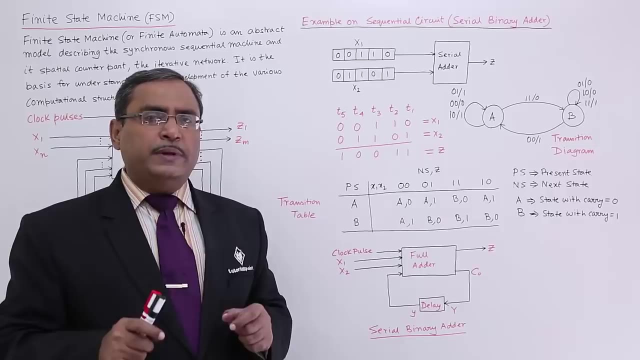 sum bit will be 0 and the state will have the carry. So I am making a transition to state b In this way. I have done. Let us take arbitrarily another one. What is b? b means I am having the carry with me. So now here, the input is 1, 1.. Then 1 plus 1 plus 1 means what? 3 means what? 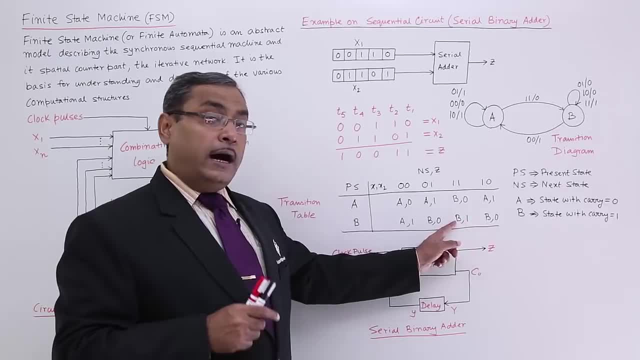 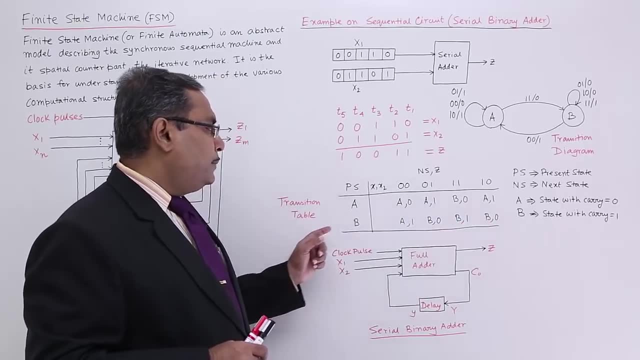 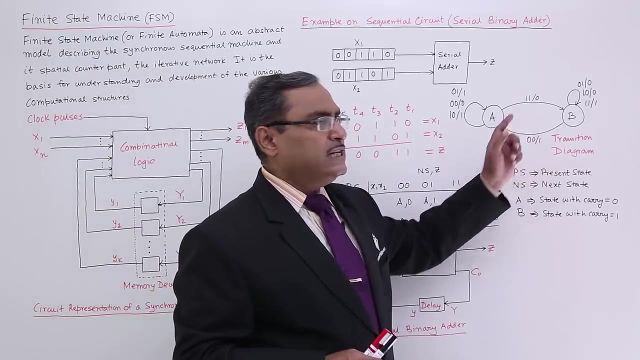 1: 1 in binary. So 1 will be the sum and I will be remaining with 1 carry. So I shall retain at my state b. So in this way this particular transition table has been formed. The similar, the same, equivalent transition system or transition diagram has been shown. 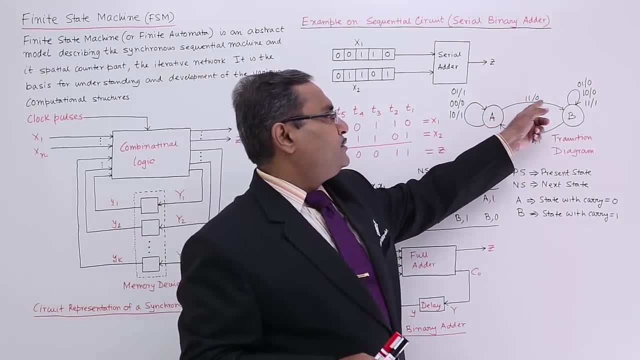 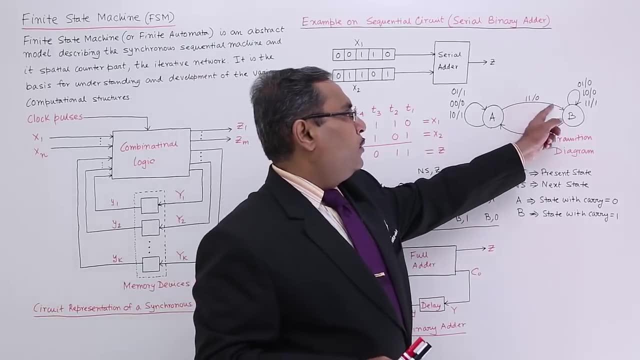 So it is my state a and this is my state b. Only here the state transition will take place. So a, a, a with input 1, 1 will have the b 0. So with 1, 1 will be going to the state b. 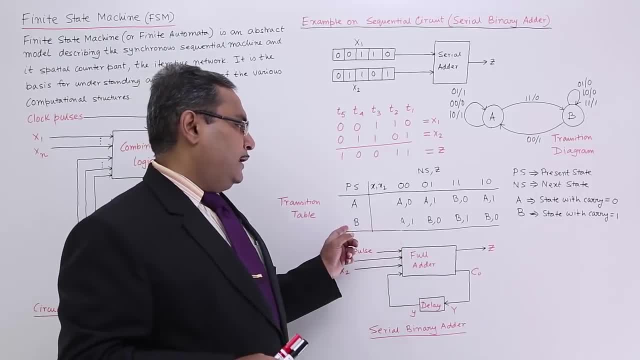 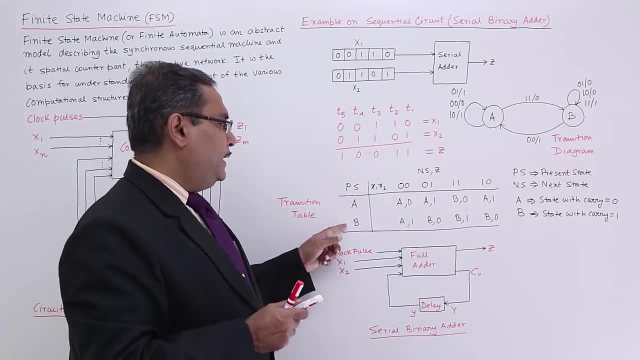 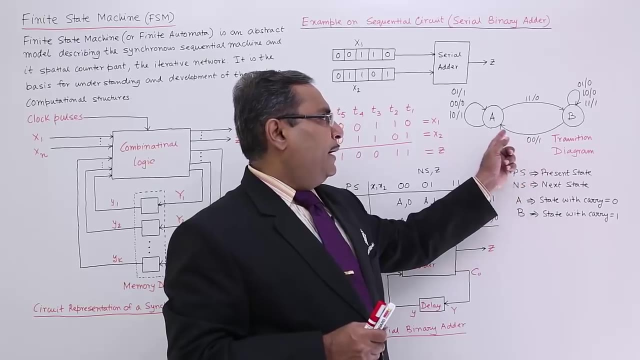 and the output will be 0.. And here also at in one state only the state transition will take place. So that is my at b: if I put 0, 0,, then my next state will be a and output will be 1.. So at state b, if I put 0, 0,, my next state will be a and output. 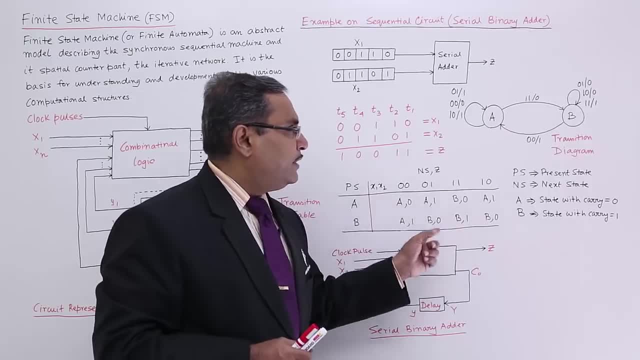 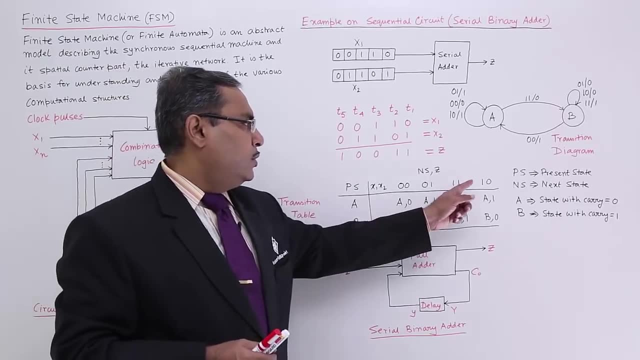 will be 1.. So in this way I have explained each and everything in the respective transition diagram. Let me show another one, arbitrarily selecting. So now a 1- 0,. next state will be a and output will be 1.. So a 1- 0.. 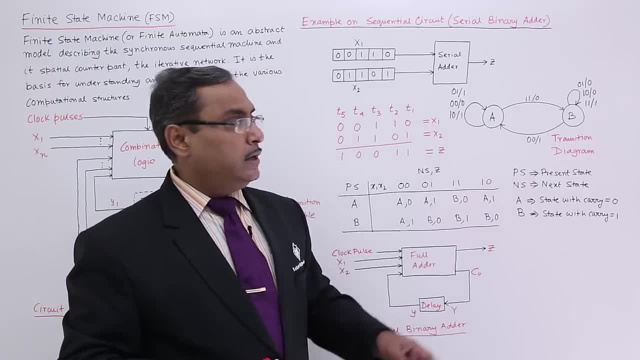 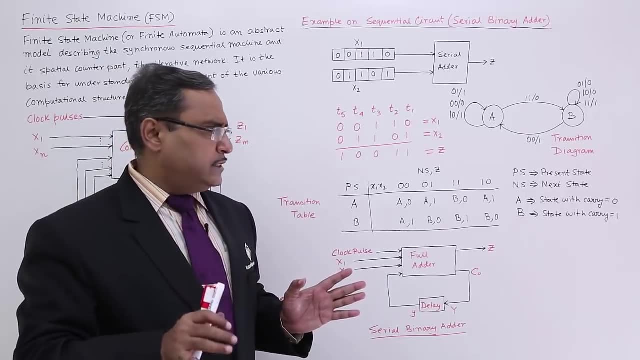 Next state will be a and output will be 1.. In this way it has been done. So this is my transition system, or transition diagram. This is my transition table. Same thing, but in two different representations. Now that is my, the basic schematic diagram of the serial adder. So 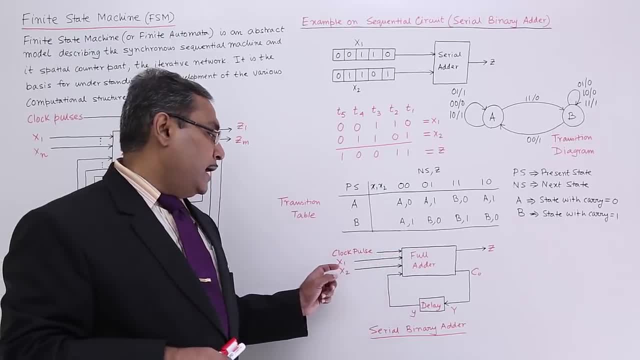 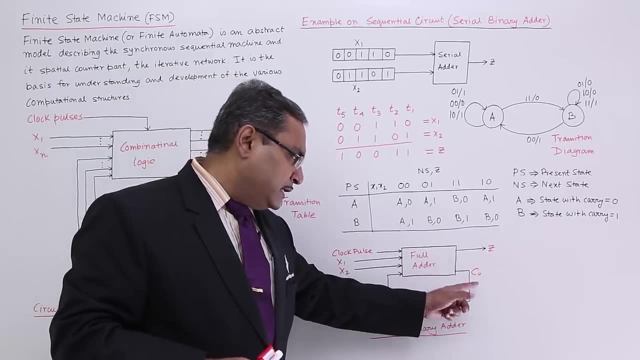 I am having this clock pulse synchronous, So that is why clock pulse must be there. And then x 1 and x 2 are. they are providing the inputs. Serial adder is getting the sum as output and the previous carry will be will become the next carry.